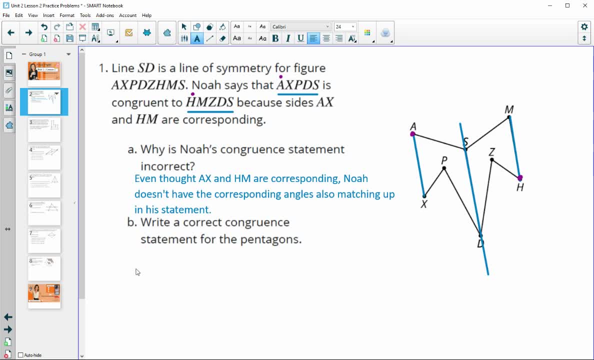 So let's continue on by keeping his statement. So he has AXPDS And we'll say that that is Congruent to And match up the vertices that way. So A actually goes with M. So A goes with M. 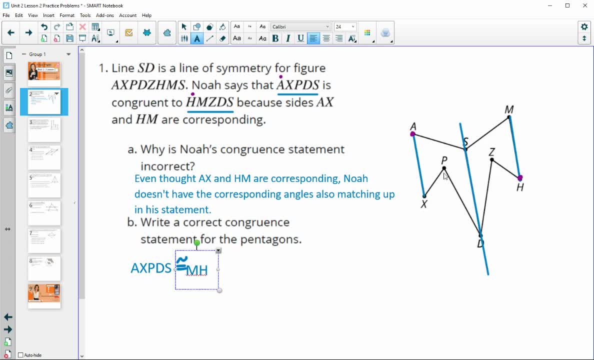 X goes with H, P goes with Z, D goes with D And then S goes with S. So this would be one congruent statement. That would be fine. You could have done other orders if you changed this first order. I'm just going to stick with his original first. 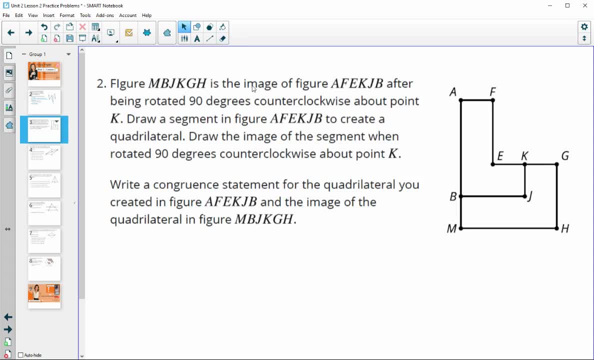 All right. number two: This figure is the image of this one, So this L shape here is the image of this L shape after a 90-degree rotation, counterclockwise, around point K. So we took it. You can spun this this way. 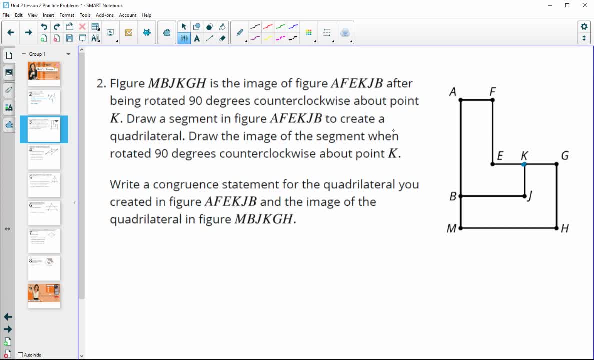 Draw a segment in figure AFEKJB, so into this one, to create a quadrilateral, and then draw the image of the segment when rotated 90 degrees counterclockwise. Then we're going to write a congruent statement. So you could do some different things here. 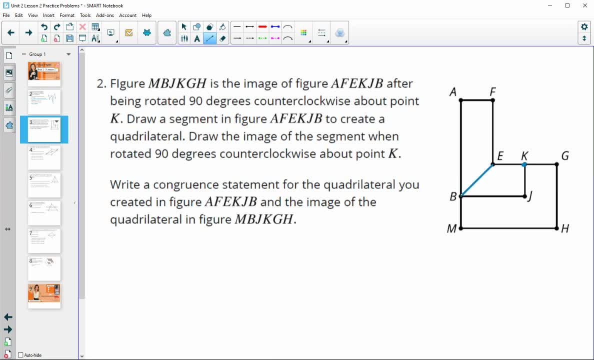 I'm just going to connect these vertices. That'll be easiest for me to replicate in the The rotated image. So EB. So when I rotate this that's going to be JH, And so then you can see that that created kind of two different quadrilaterals. 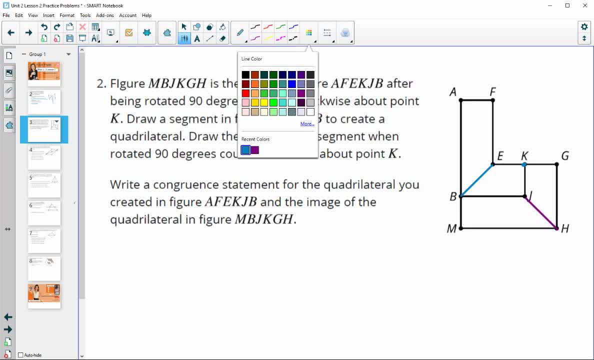 So whichever one you would like to use in writing, your congruent statement would be fine, So I'm going to go. ABEF for mine Is congruent to. So now A in this new shape. So here's the one we just looked at. 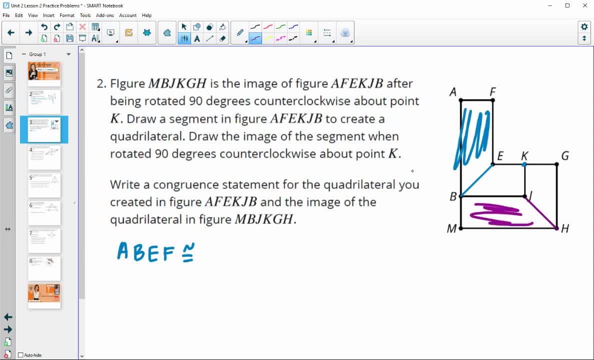 And now we're rotating it to this one. So A is going to rotate to M, B is going to rotate to H, E is going to rotate to J And F is going to rotate to B. So that's one option you could have ended up with there. 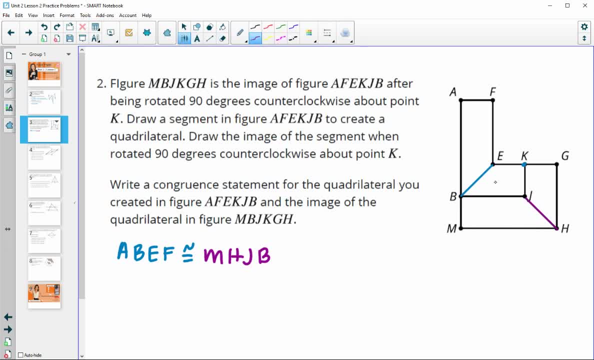 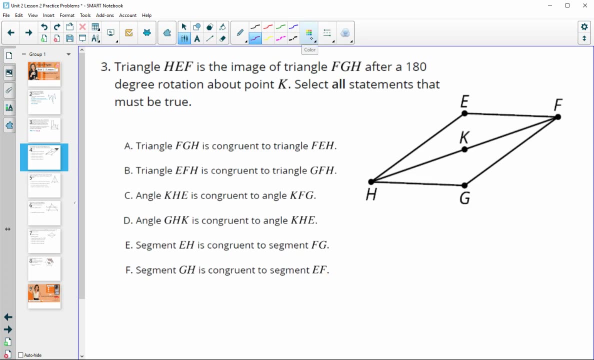 Could also have used With this same segment. you could have used this shape to this shape as well. So there's some different things possible there, But there's one example. Number three, triangle HEF, is the image of triangle FGH after a 180 degree rotation around point K. 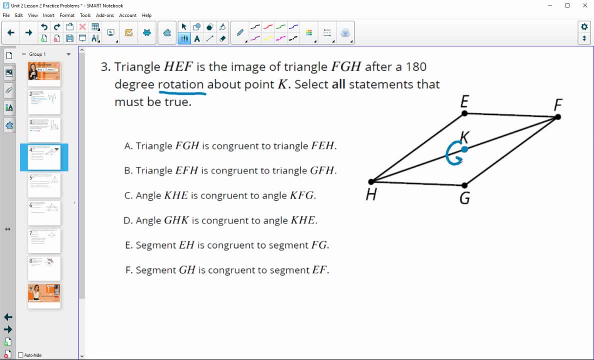 So here's the rotation point. So we're rotating around: Select all statements. that must be true. So we've got a rotation and we want to select all statements. So let me see if I can get this to rotate on here, See if we'll be able to kind of show what the rotation looks like. 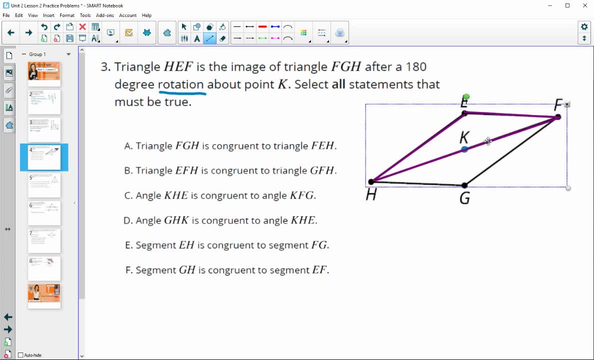 All right, So when we rotate it'll be like that: Whoops, Okay, So rotating 180 degrees, So you can kind of see then how F in the top triangle is going to rotate to H in the bottom triangle. Okay, 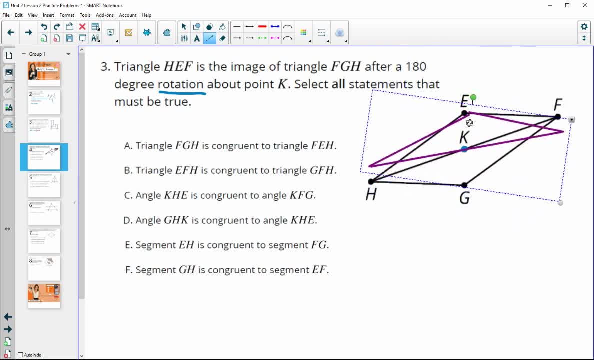 E will rotate to G And H in the top will rotate to F in the bottom. So that kind of gives you a visual of watching what's happening with those coordinates, What's happening with those corresponding pieces. So let's take a look here. 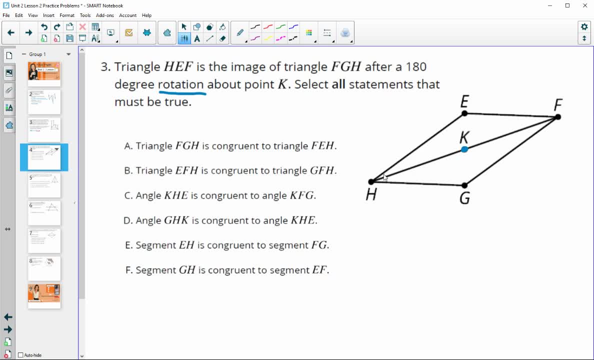 So this one says triangle FGH is congruent to FEH, Which is not true because, remember, we need to match up the corresponding vertices. So if we look at FGH, Okay, This angle, This angle F in the first triangle, needs to match angle F. 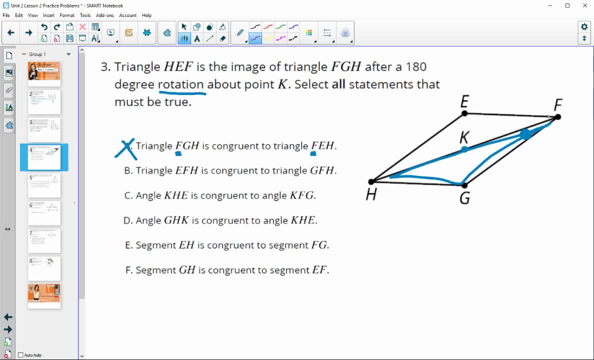 In this second triangle And it does not. Okay, These two angles are not congruent. F rotated down to H, All right. Then the next one says that triangle EFH- Okay, So EFH is congruent to triangle GFH. 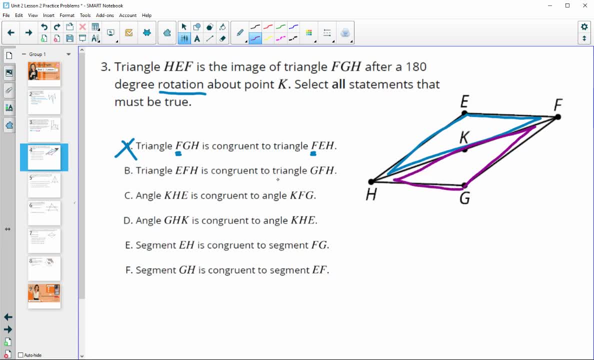 So E and G are corresponding, So that's fine. So this E with G is fine. But F in these two triangles are not congruent, So we can't match up F with F. So that's going to be false Angle KHE. 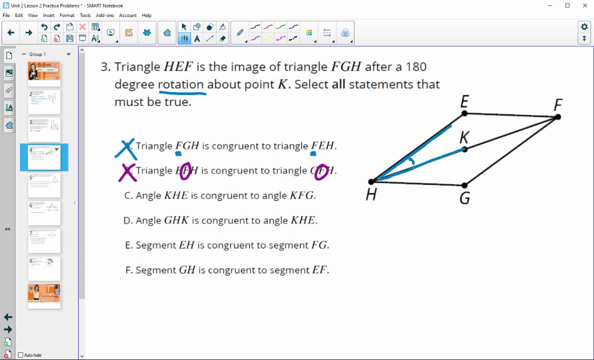 So here's KHE. So this angle here is congruent to KFE. So KFG, This angle here, That is true: H on the top rotated over onto F on the bottom. So that is true GHK, GHK is this angle here. 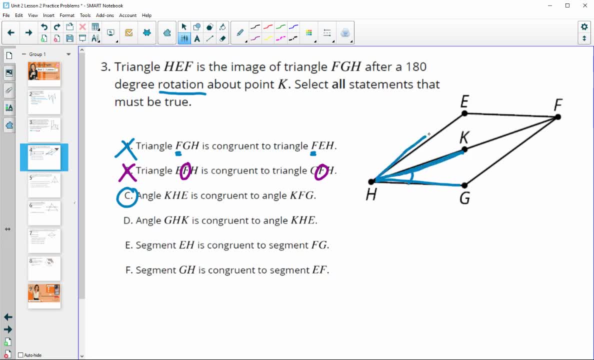 Is congruent to KHE. That is false. Okay, This little H rotated over to here, So we've got kind of alternate interior angles when we're looking at rotations. If this were a reflection, if this line was the line of reflection, then these two little angles next to each other would be congruent, but not in a rotation. 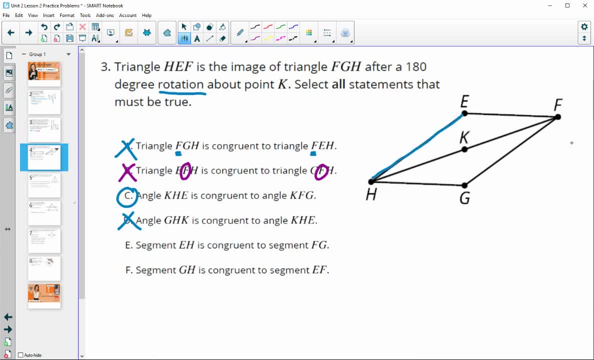 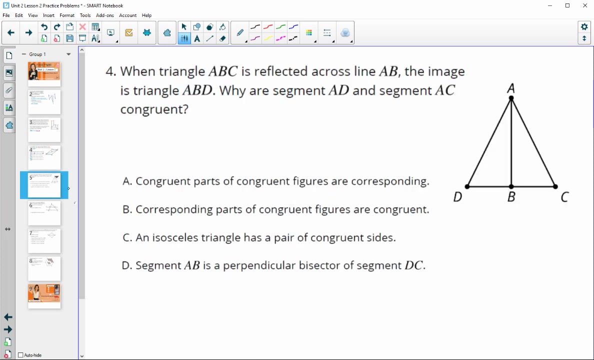 Segment EH is congruent to segment FG, That is true. Okay, This will rotate all the way over to there. And then, finally, GH is congruent to EF, And that is true as well. Number four, When triangle ABC is reflected across line AB. 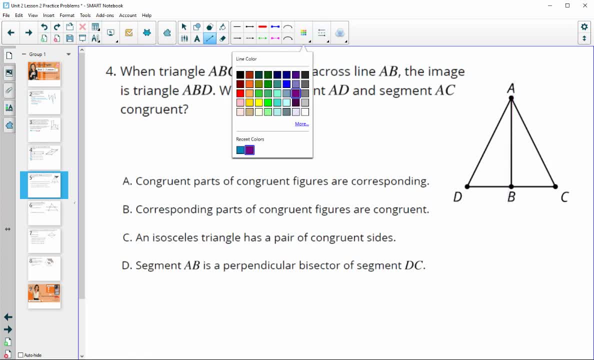 So now we're doing a reflection over this line. Let me maybe do that blue, It's easier to see. Okay. So now we're reflecting over this line: Why are segment AD? Okay, So why is this segment and this segment AC congruent? 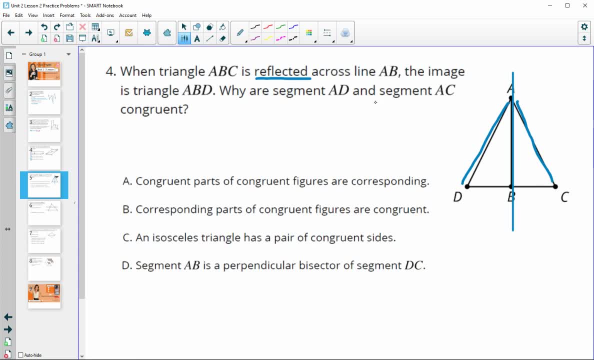 So why are they congruent? What would be the justification? So remember, when we're reflecting, we're taking this triangle here, So ABC, So we started with this, and then we're just reflecting it over this segment. So congruent parts of congruent figures are corresponding is not accurate. 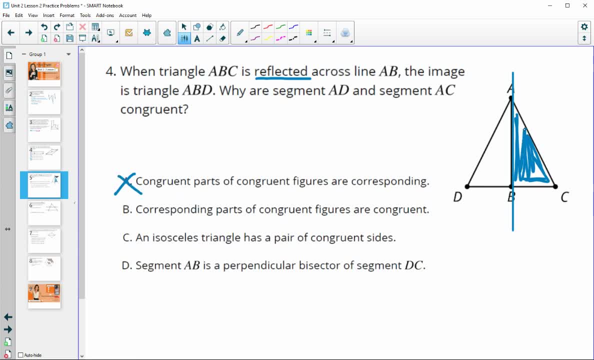 Corresponding parts of congruent figures. So a reflection definitely creates congruent figures. So when we reflect we know that this is a congruent figure to the original And then we also know that this segment is corresponding to this one. So they are corresponding parts of congruent figures. 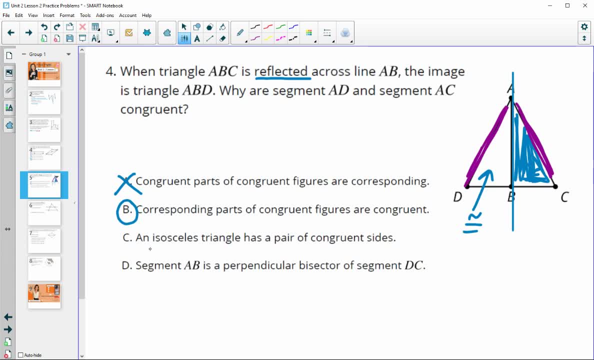 So they're going to be congruent to each other is true, And isosceles triangle has a pair of congruent sides. That's true, But we did not start with an isosceles triangle, So nothing in here told us that we started with isosceles. 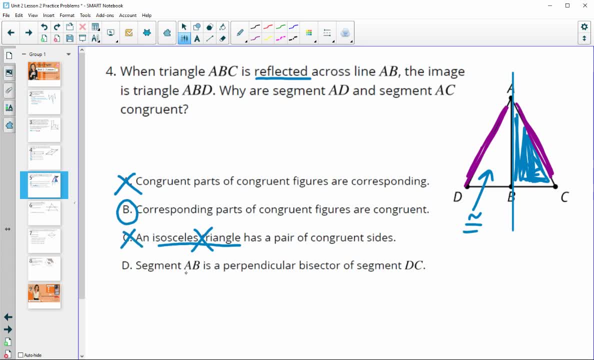 So that's why that one's false. And then segment AB is the perpendicular bisector of DC. It is after the reflection It does become the perpendicular bisector, But they never told us anything in here about a perpendicular bisector, So it's not the justification for this problem. 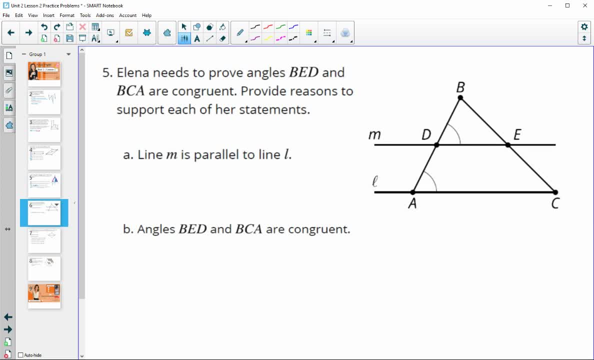 Number five: Elena needs to prove that BED and BCA are congruent. So BED is this angle here, And then BCA is this angle- Provide reasons to support her statements. So her first statement is that she knows that M is parallel to L. 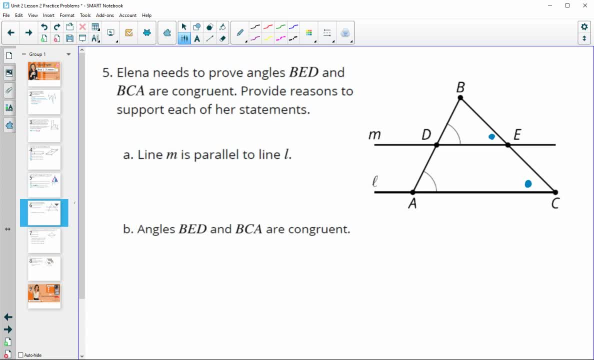 How does she know that? So she knows that M is parallel to L because of these two angles that are congruent. So these two angles that are congruent are corresponding angles, And when corresponding angles are congruent, then we know that the lines are parallel. 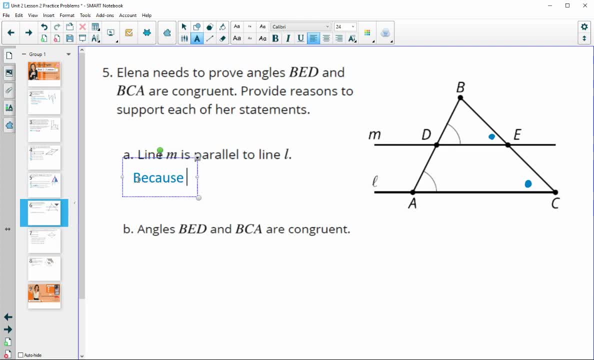 So the lines are parallel because angle BDE and angle BAC are corresponding. So she knows it, even because we have the corresponding angles that are congruent. So the lines are parallel, All right. And then how does that help her? So now that she is justified that these two lines are parallel because of corresponding angles being congruent, 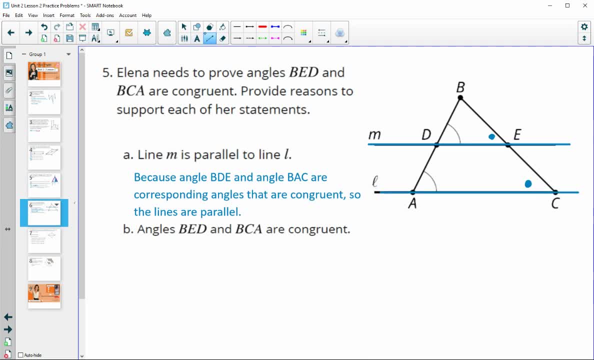 Now that we know the lines are parallel, now we can say that these two are congruent because they are corresponding angles. So BED and BCA are congruent because they are corresponding angles created by two parallel lines and a transversal. So then they're congruent. 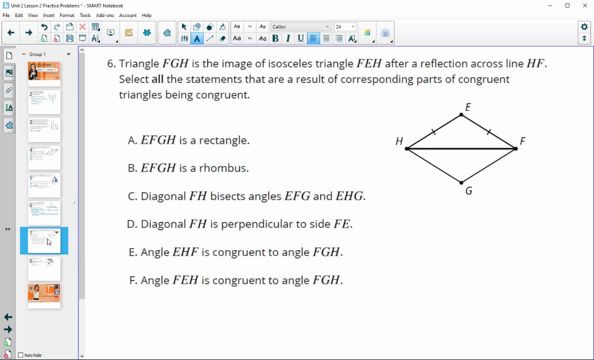 Number six, triangle FEH is the image of isosceles. triangle FEH after a reflection across the line FH. So we've got a reflection Over this line. select all statements that are the result of corresponding parts of congruent triangles being congruent. So EFGH is a rectangle. That's not true. We don't know anything about. 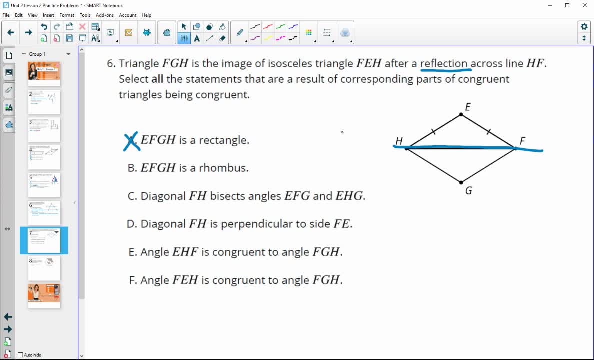 90 degree angles to give us a rectangle. FEGH is a rhombus, So remember, rhombus means that we have four congruent sides And so, since we know that these two images are congruent, we can say that these two images are congruent. So EFGH is a rhombus. 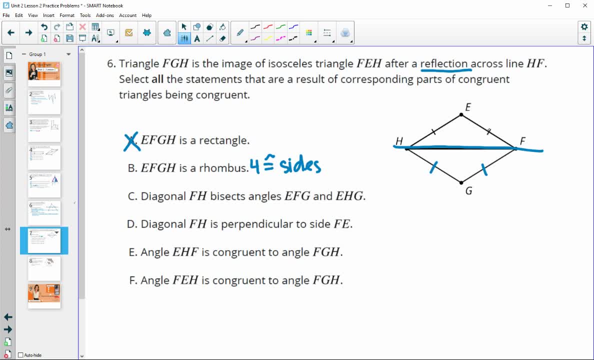 We know that this side and this side would also be congruent to these ones. So all four are definitely congruent. So this is true: Diagonal FH bisects angle EFG. So here's EFG and angle. So we're saying this angle is equal to this angle And it's saying that it bisects angle EHG. 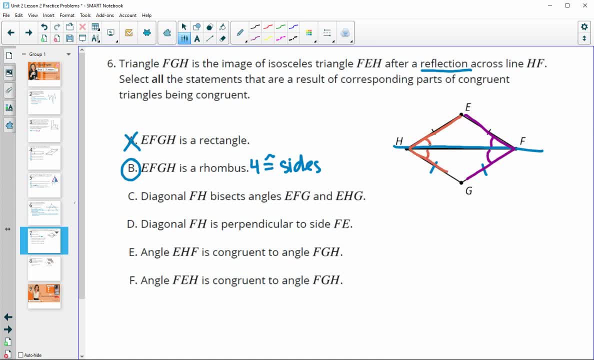 So this one, And that is definitely true. We know that these two angles are congruent to each other and that these two are congruent to each other with that reflection because of the corresponding parts. So this is true. Diagonal FH is perpendicular to side FE. 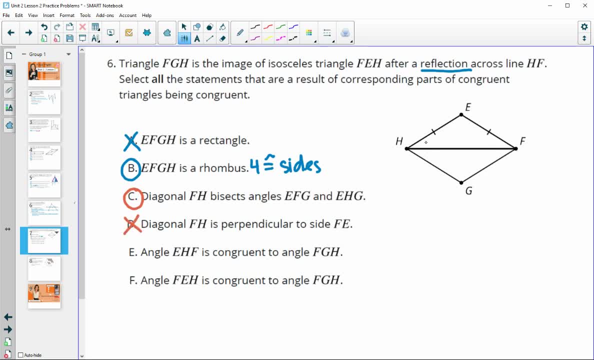 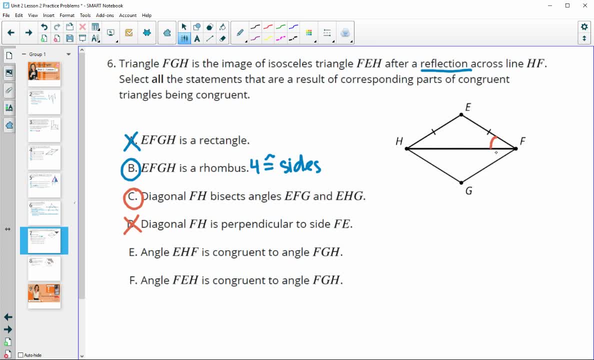 So angle HFE. this angle here is congruent to FGH. FGH is this one, Those are not corresponding parts. So that is false. And then, finally, angle FEH. So FEH is this one- is congruent to FGH. This one, Those are definitely corresponding parts of congruent. 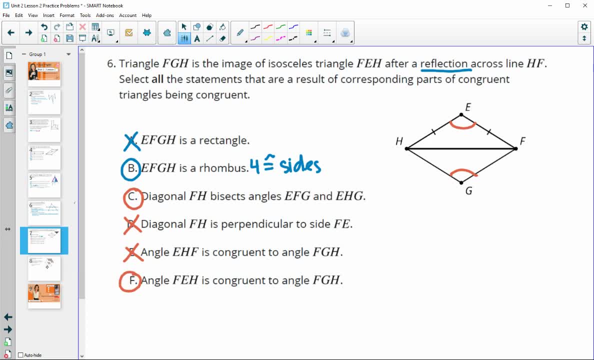 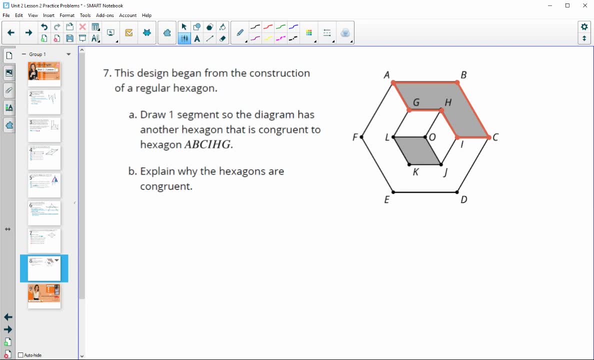 triangles. So that is true. All right, then number seven: this design began from the construction of a regular hexagon. Draw one segment so that the diagram has another hexagon congruent to the one highlighted here. Explain why the hexagons are congruent. So let's draw another line in here. 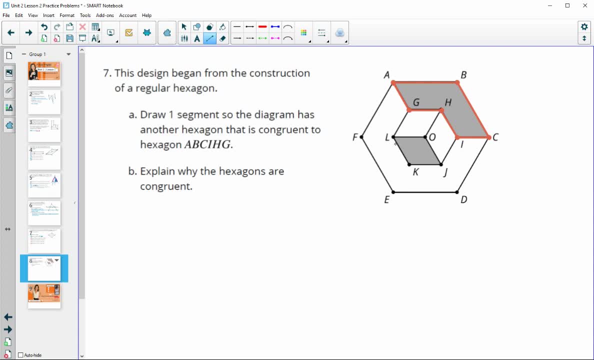 to make a hexagon congruent to that one. So we kind of need like two chunks of this. So here's one, two chunks. So I'm going to draw my segment here and that's going to actually create two congruent hexagons to that, And so now explain why the hexagons are congruent. So we know. 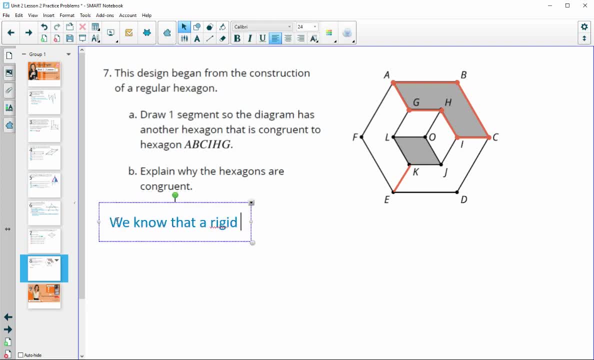 that a rigid motion- um, um- takes a figure onto a congruent image, And um, so we can see that this we could rotate. So one of the rigid motions that we've learned about is rotating Um, and so we can see that we could rotate this onto. 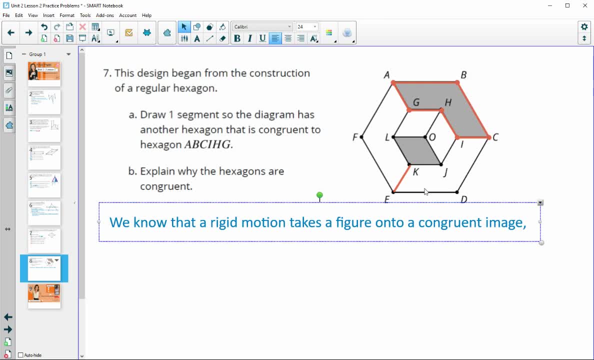 this image, or we could rotate it this way to this one, And so we know that a rigid motion takes a figure onto a congruent image. and if, if, if, if we rotate um abcihg by 120 degrees And you can pick clockwise or counterclockwise. 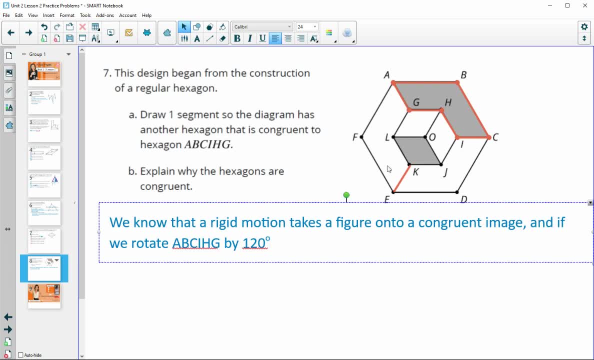 It actually doesn't matter this time, Because if you do counterclockwise, you'll land on this one, And if you do clockwise, you'll land on this one. Um, so if we rotate a abcihg by 100 degrees counterclockwise-